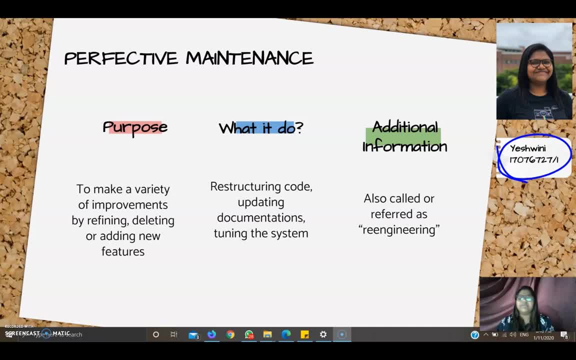 by restructuring the code, updating the documentation, tuning the system and so many things more, And it's also called as re-engineering, So it focuses on the evaluation of the requirements and features that existing in the system As the user interacts with the application. 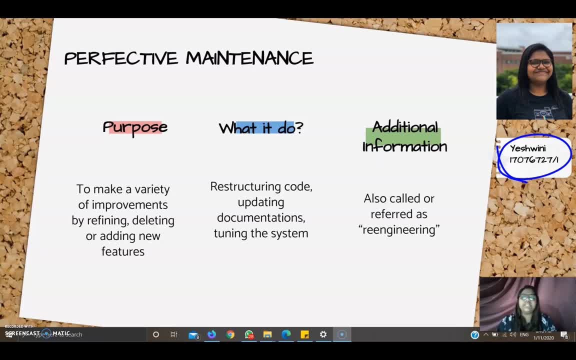 they may notice things that you did not do or suggest new features that they would like to be part of the software. They may notice things that you did not do or suggest new features that they would like to be part of the software Which could become the future projects or enhancements. 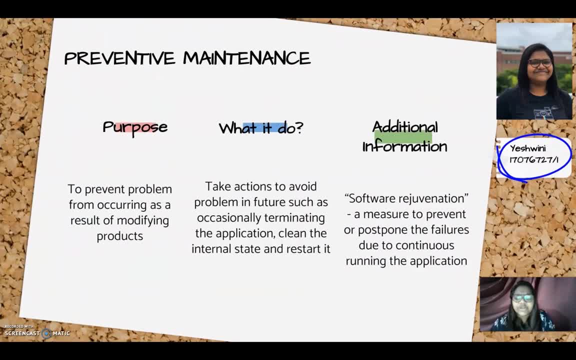 Moving on to the second one, which is perfective, I'm sorry, preventive maintenance. So the purpose is to prevent the problem from occurring as a result of modifying products by taking actions to avoid problems, in such as occasionally terminating the application, clean the internal. 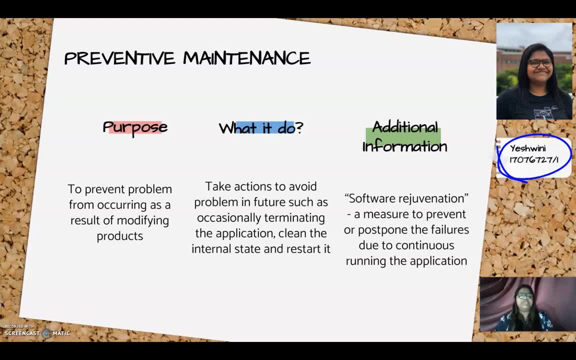 state and restart it. So it helps to make changes and adaption to the software so that it can work for a very longer period of time And it's also to prevent the deterioration of the software. and it can change. Additional information is a software- rejuvenation- It's also called a software. 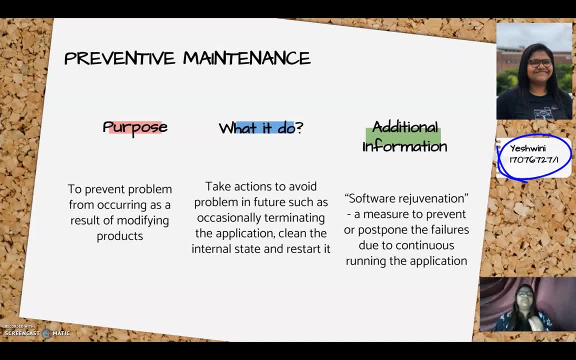 rejuvenation, which is a measure to prevent or postpone the failures due to continuously running the application. For all the business and organizations, preventive maintenance is essential part of the software development cycle. It's not something that one can skip or avoid. It's absolutely necessary for the success of the software and evaluation into the future. 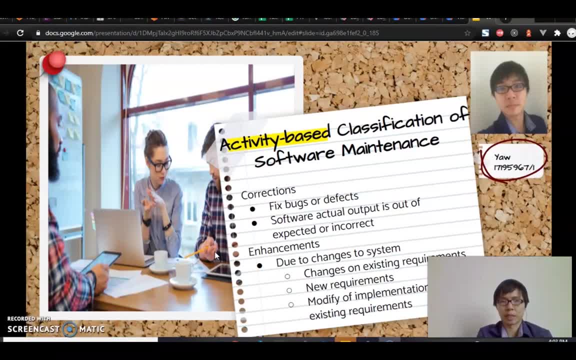 Today I was going to present on the activity-based classification of software maintenance. We can classify the software maintenance to two types of category of activity. The first one is the correction activity and the second one is the enhancement activity. So when we deploy a software to a production level and then it will be, 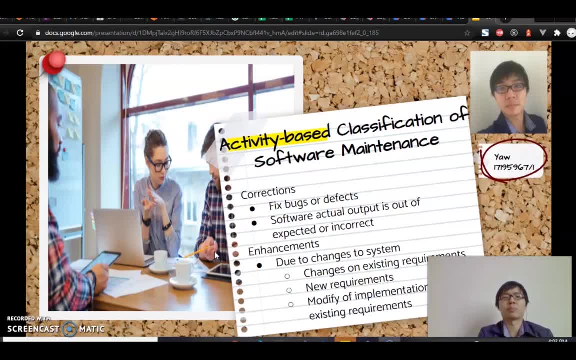 using by different kind of end user. So when they are using the application or the software there will be bugs or defects. that happen. So what we will do during the correction activity is to correct this type of unexpected output that happens to the software. 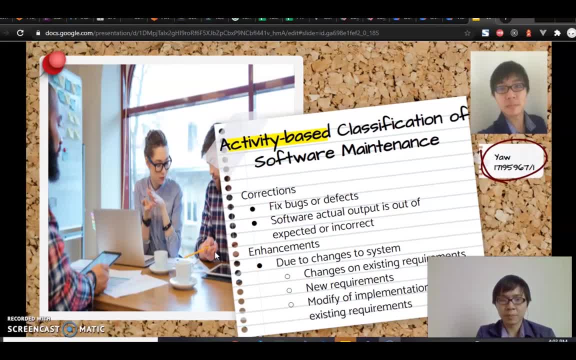 So the second one is to enhance the enhancement activity. So this is the enhancement activity. So this enhancement activity is caused due to the changes to the system. So there will be different kind of changes that we can sub-characterize, which is the change on the existing requirements and also some changes to the system, which 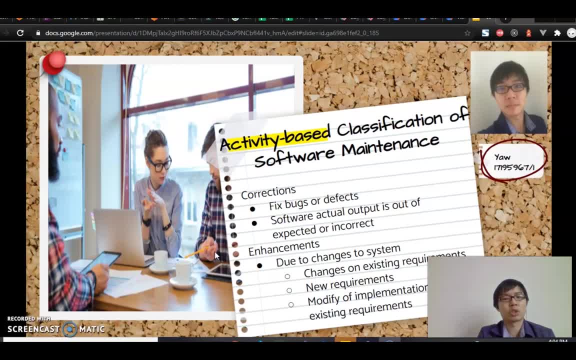 introduce a new requirement to the system, And then the last one is the modify of the implementation of the existing requirement, And then this will not change on the requirement itself. We just change the pattern of the implementation that we do. In other words, it's changing on the source code as well. 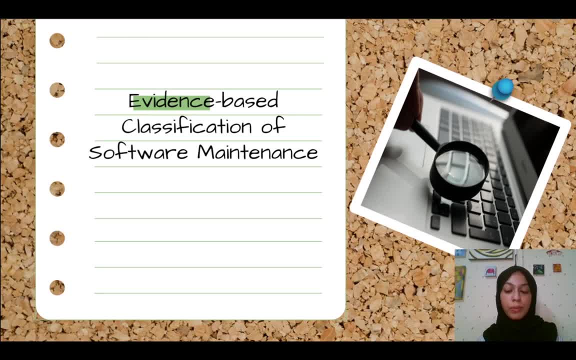 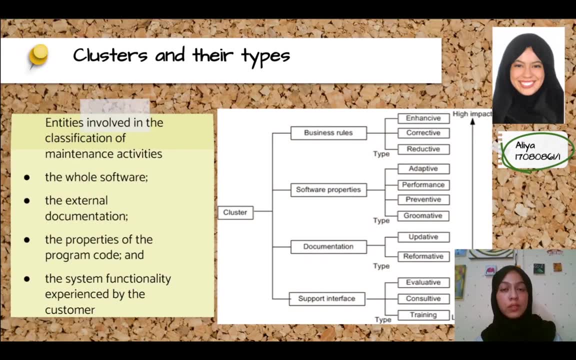 So that we're presenting on the implementation of the system. So we're presenting on the evidence-based classification of software maintenance. So evidence-based classification is the further refined version of the intention-based classification, by basing the classification on objective evidence that are measured through. 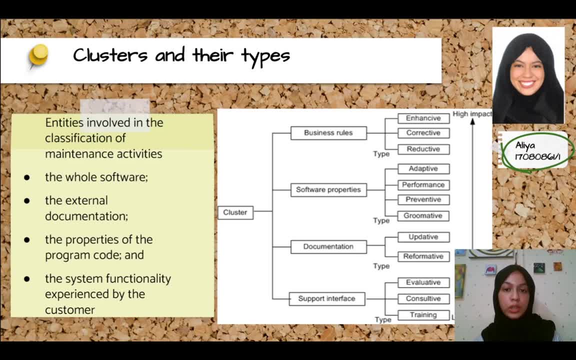 observations and comparisons of the software before and after modifications. There are four entities involved, which are the whole software, textional documentation, the properties of the program code and the system functionality and the customer experience. So there are four clusters. The first one is the business rules. It consists of three types, which is the 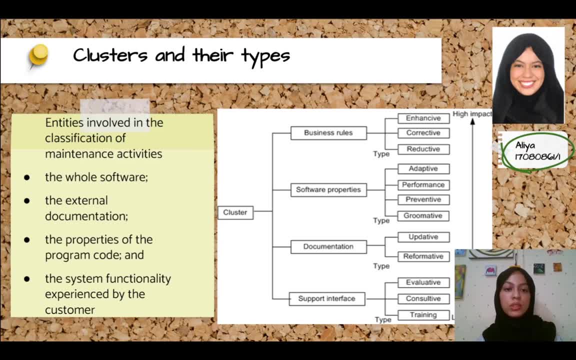 Enhance, Correct and Reductive. The business rules cluster involves the user and the business level functionalities. The second cluster is the software properties cluster, which consists of adaptive, performance, preventive and gummative. The software properties cluster is concerned with 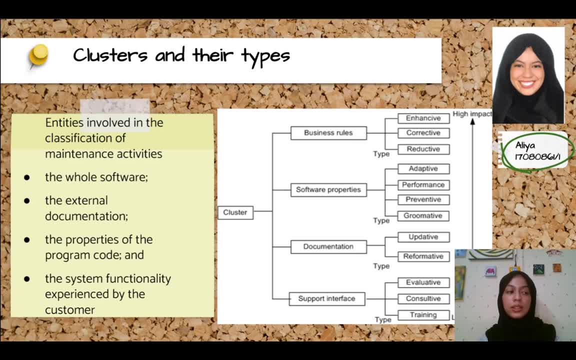 the modifications in the attribute of the software. that doesn't involve the modifications in the system functionality delivered by the system. The third cluster is the documentation cluster. It consists of update and reformative. The documentation cluster is concerned with the modifications in the documentation which does not include the source code. 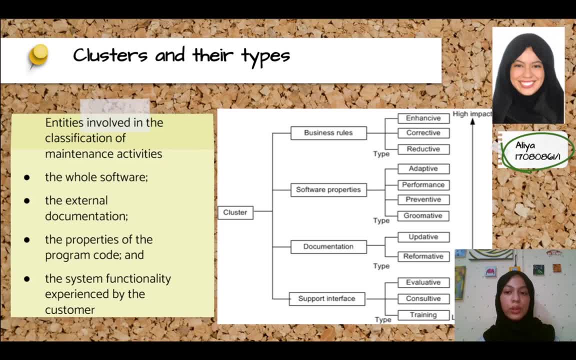 The last cluster is the support interface cluster. It consists of evaluative, consultative and training. This cluster relates to the modification on how service or maintenance personnel interact with the stakeholders and customers. It is the programming that preserves information and enables the user to understand the system. 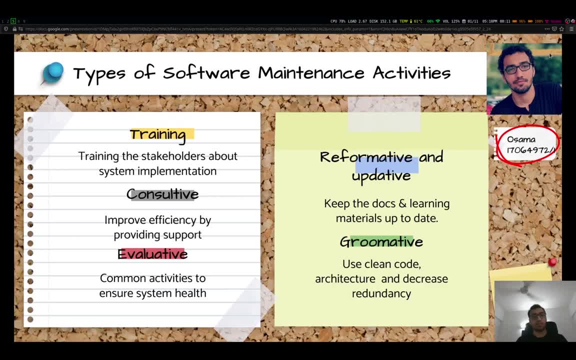 as well as the participants. One of those activities to start with is the training�م sort of stakeholders. It is a training activity where we teach the stakeholders how the system works or the system implementation overall. The second one is the consultative activities, which aim to provide. 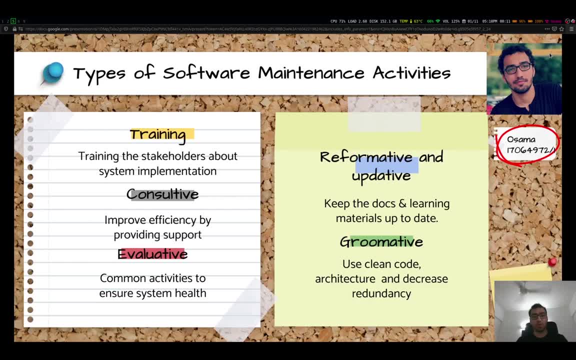 support or a kind of help desk for customers to overall improve efficiency. The third is the evaluative activities, which includes reviewing the program code and its design if it is up to date with the changes in the code of the system. The third is the evaluation activities, which include: 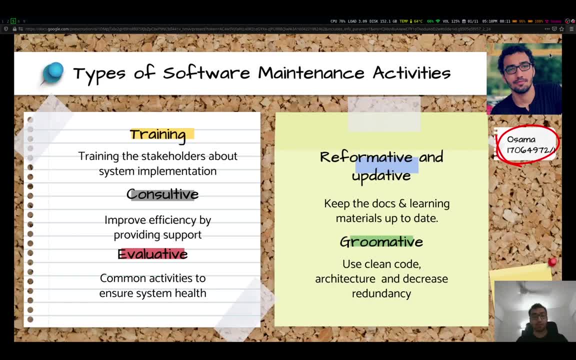 reviewing the program code and its design if it is up to date with the changes in the code of the system. and, ultimately, the evaluation of the program code or the implementation of the program code To not designed, tests and executed and more the fourth and fifth activities that mainly focus: 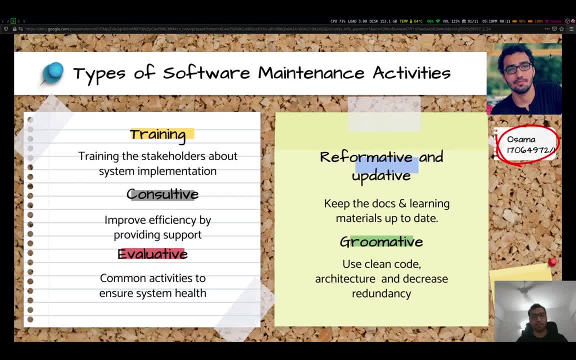 on the docs, which is the reformative and updated activities. it's it's mainly to keep the docs up and up to date with also the learning materials and while maintaining readability of that docs as well. the sixth one is the chromatic activities, which aims to simplify the code more. 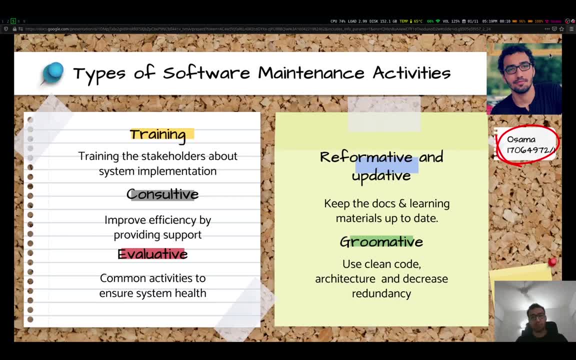 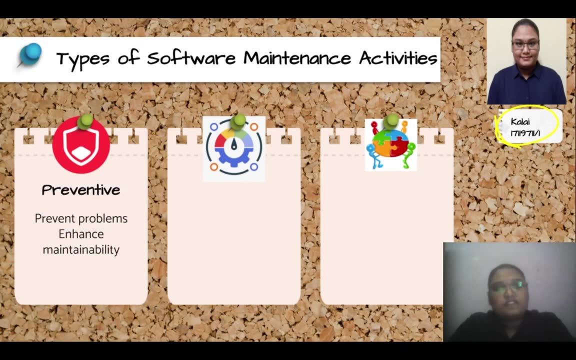 and use more efficient algorithms, if it's possible, better naming conventions, uh, enforce some clean code, some key architecture, while making up-to-date backups of the system. i'll be talking about the other types of software maintenance activities, and the first one will be preventive. preventive is all about preventing a problems to enhance maintainability, for example, in a food delivery. 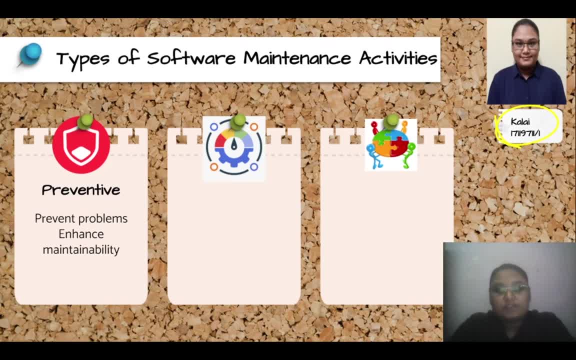 system. it should be reflected or update from time to time so that it won't become a legacy system. and the next one is performance. performance is where a system should have a fast response time. for example, a invoice should be generated as soon as a customer place and order. and the next 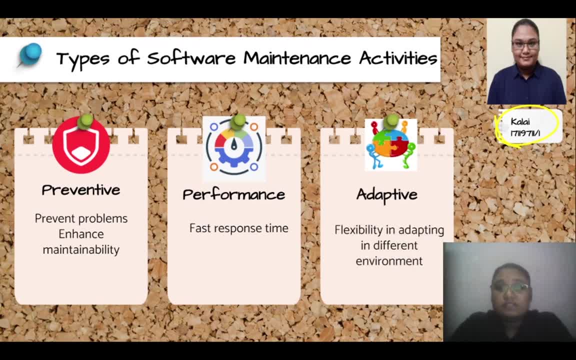 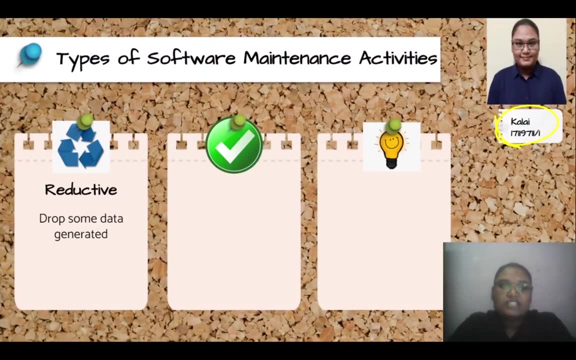 one is additive. additive is where a system should be able to adapt in different environments. for example, a food delivery system should be able to run in both web application and mobile application without any problem. and the next one is reductive. reductive is where some generated data are dropped. and the next one is corrective. corrective is where all the 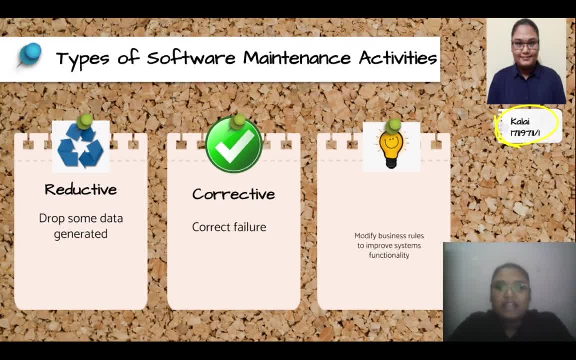 bugs and failures are corrected from time to time, and the last one is an unsave and i think, where your business rules are modified so that it can improve the system functionality. for example, a new feature can be added into a food delivery system so that so that more user can use the app without 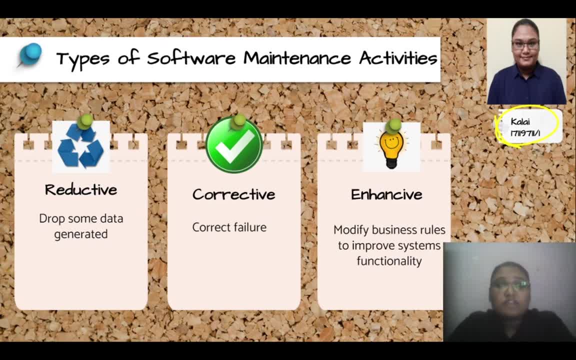 any problem. so as a whole, there are 12 types on the map if you use the apps los statot neighborhood plus direct flow system, for example. for example, there are dimensionally way for yes and a wide 12 types of software maintenance activities, which can be grouped into 4 main clusters.